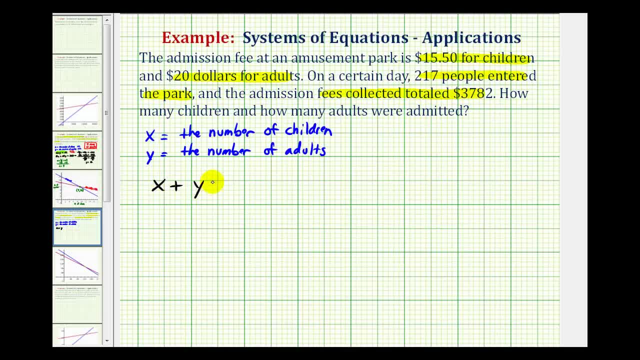 this tells us that x plus y must equal 217.. And then again, every child has to pay $15.50 and every adult has to pay $20.. Resulting in a total of $3,782.. Which means 15.50, or just 15.5 times x. this is the amount of money collected from the children. 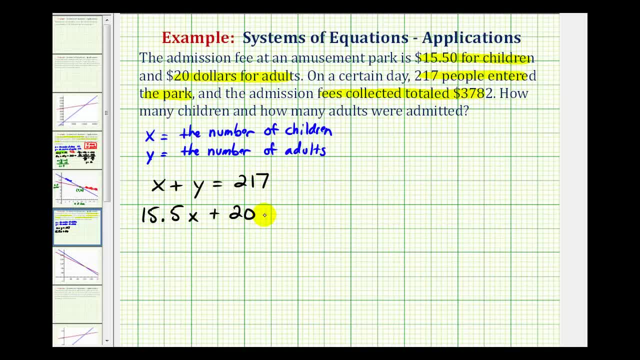 plus $20 times y- this is the amount of money collected from the adults- must equal $3,782.. So this is our system of equations. If we want to solve this algebraically, we can use the substitution method Or the elimination method. 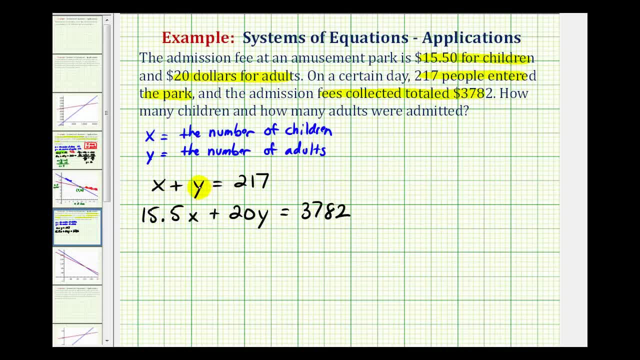 Since we can solve this first equation here pretty easily for x or y, I think we'll use the substitution method. So if we subtract x on both sides of this first equation, we can rewrite this as y equals 217 minus x, And now we'll use this equation and perform substitution into the second equation. 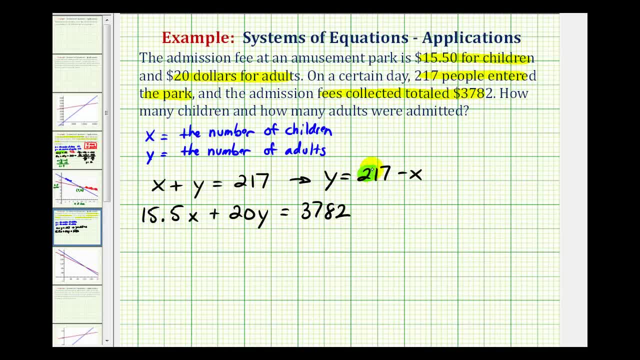 Since y is equal to 217 minus x, we can substitute or replace this y here with 217 minus x, And this will give us an equation with one variable and therefore we can solve for x. So we'd have 15.5x plus 20 times 217 minus x. 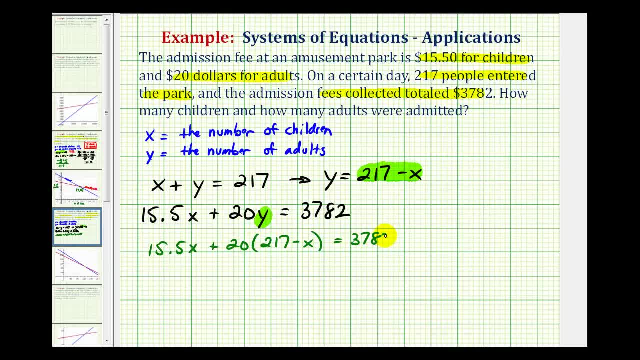 must equal 3,782.. So now we'll clear the parentheses and solve for x. So we'll have 20 times 217, that's going to be 4,340, minus 20x must equal 3,782.. 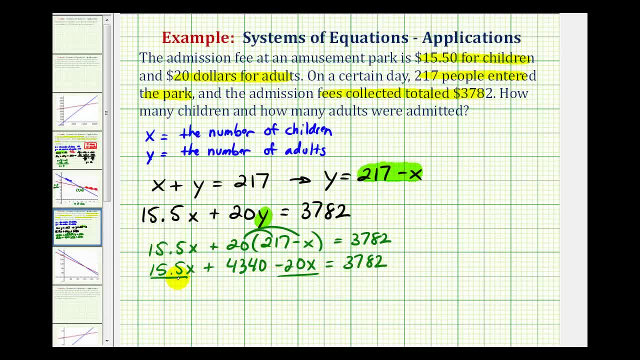 Let's combine our like terms here and here: 15.5x minus 20x is going to be negative 4.5x. Now we'll subtract 4,340 on both sides. This would be zero, so we have negative 4.5x. 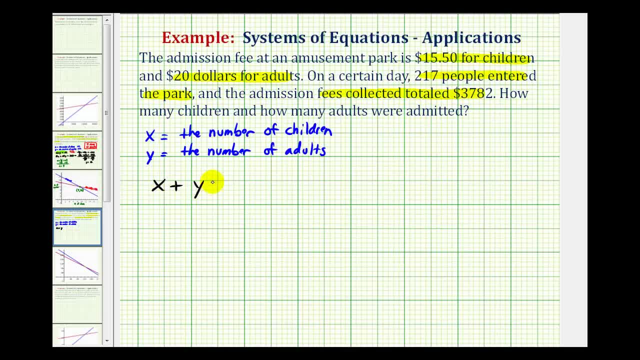 this tells us that x plus y must equal 217.. And then again, every child has to pay $15.50 and every adult has to pay $20.. Resulting in a total of $3,782.. Which means 15.50, or just 15.5 times x. this is the amount of money collected from the children. 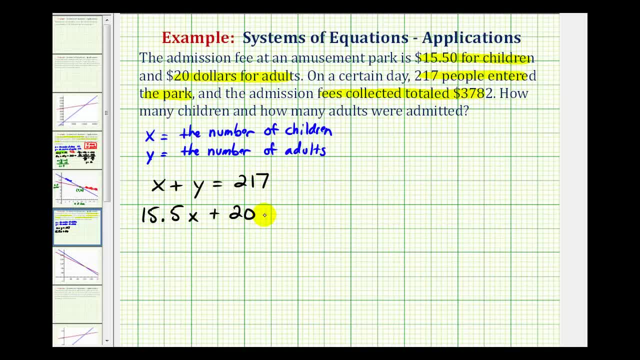 plus $20 times y- this is the amount of money collected from the adults- must equal $3,782.. So this is our system of equations. If we want to solve this algebraically, we can use the substitution method Or the elimination method. 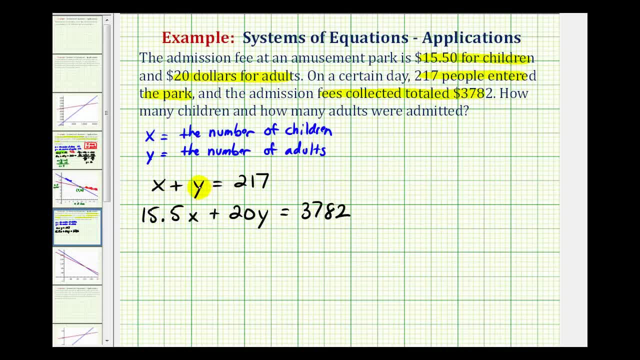 Since we can solve this first equation here pretty easily for x or y, I think we'll use the substitution method. So if we subtract x on both sides of this first equation, we can rewrite this as y equals 217 minus x, And now we'll use this equation and perform substitution into the second equation. 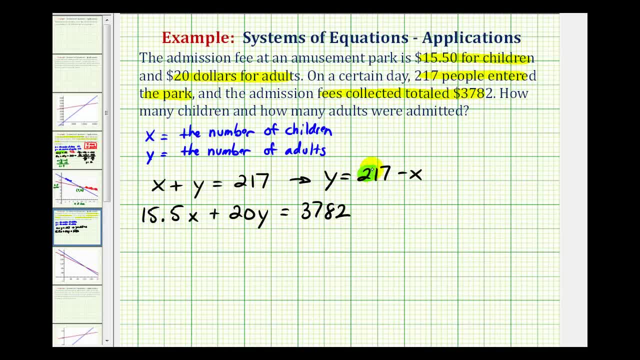 Since y is equal to 217 minus x, we can substitute or replace this y here with 217 minus x, And this will give us an equation with one variable and therefore we can solve for x. So we'd have 15.5x plus 20 times 217 minus x. 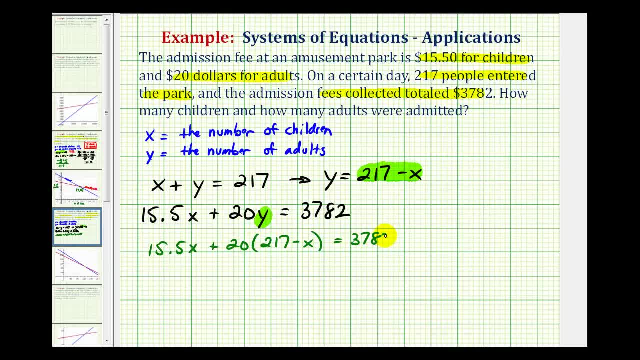 must equal 3,782.. So now we'll clear the parentheses and solve for x. So we'll have 20 times 217, that's going to be 4,340, minus 20x must equal 3,782.. 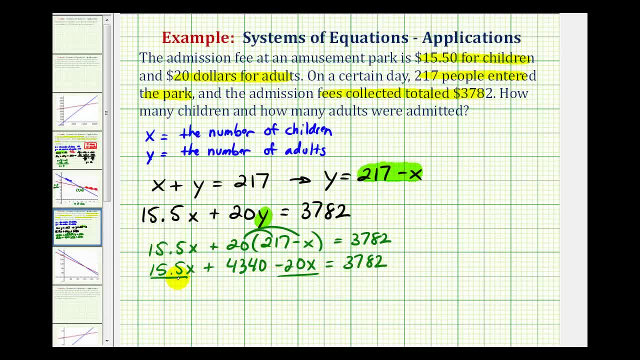 Let's combine our like terms here and here: 15.5x minus 20x is going to be negative 4.5x. Now we'll subtract 4,340 on both sides. This would be zero, so we have negative 4.5x.